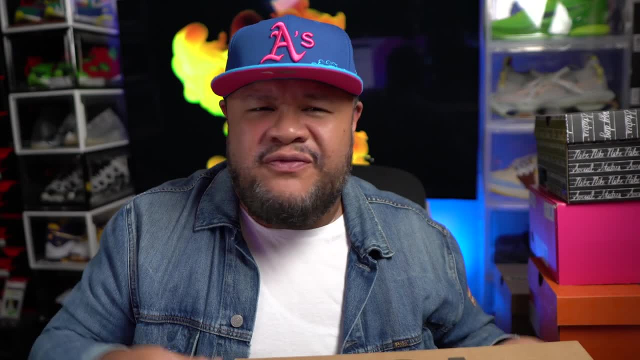 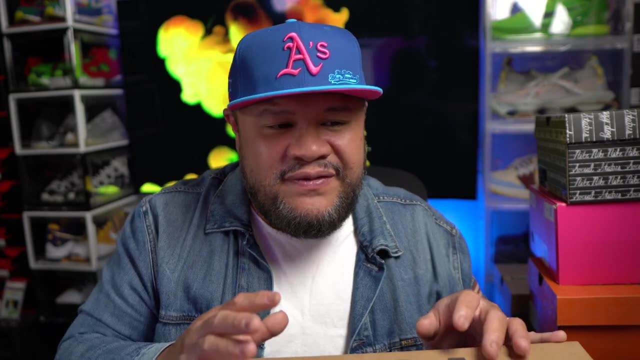 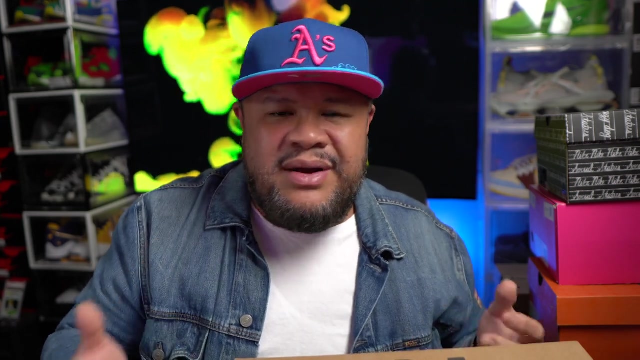 there's some truth to that, because I ended up the first drop of the day was the Utility Black 450.. Now I already have the slate, the dark slate 450s, And I did not happen to pull it out before the drop. And then I think they said the only difference was the heel had a brown hit on. 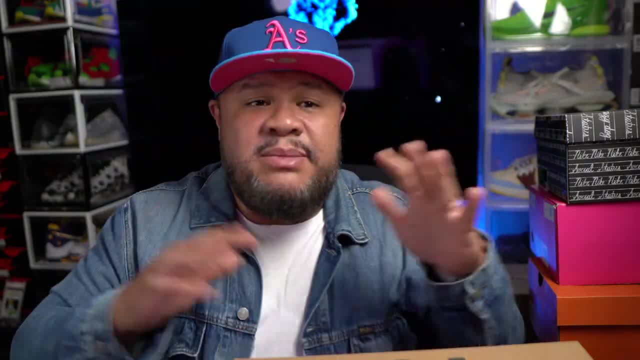 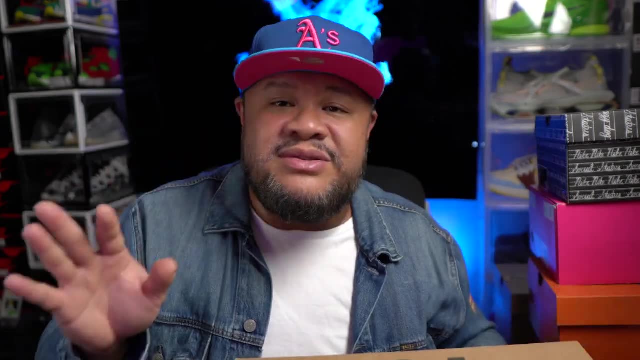 it And I was like: nah, I can't be. These Utility Blacks got to be darker, They got to be darker, And I just got the shoe today, Very fast shipping, Indeed, I'll give you that much. Some of your models suck, besides Yeezy. 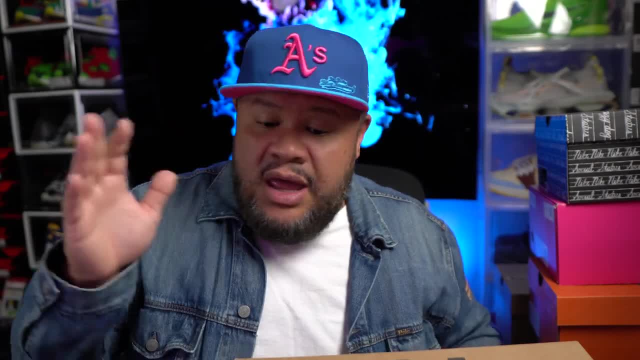 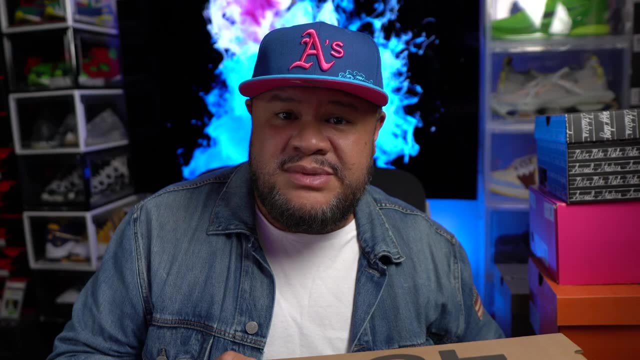 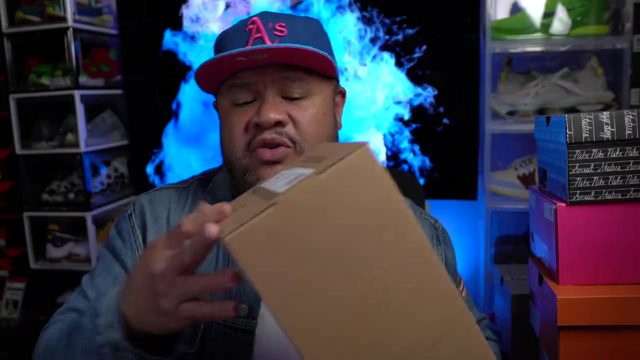 But you do ship fast, All right. And yeah, Kanye, Kanye, I got a lot. I got another video on Kanye coming up of how he stole some designs, But here's the shoe. I looked at these real quick before I got it. So I always go size 13 on these I've bought. I've actually worn my gray ones. I. 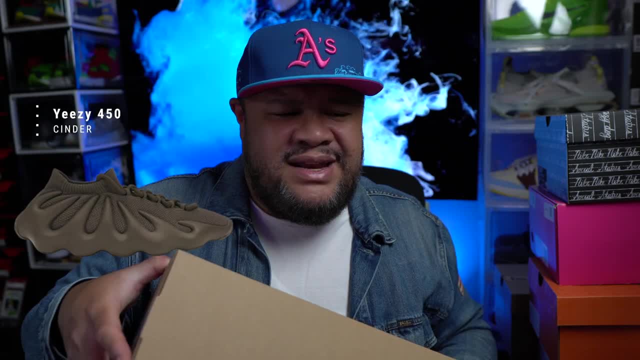 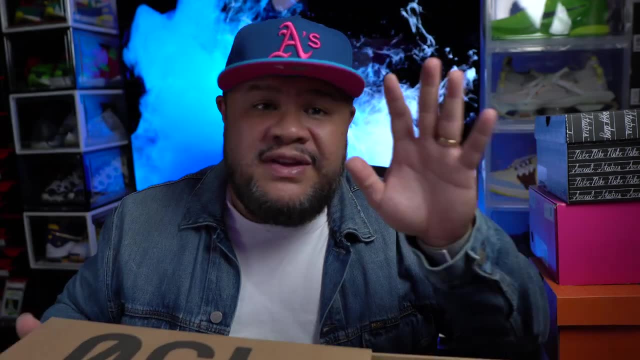 forgot what they're called. I don't know what color they are. I wore the gray ones And I have two pairs of the green ones which, which I don't know why, how, how, I got two pairs, I don't know, But I was going to pull one of each. 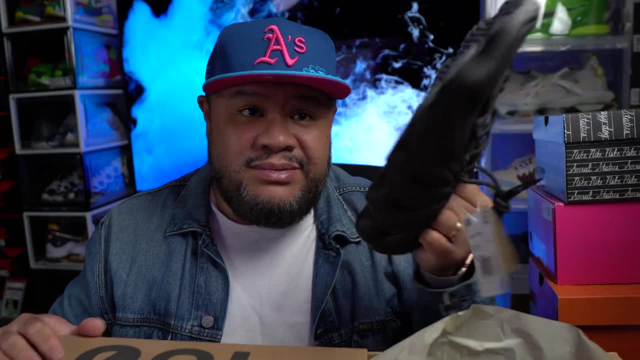 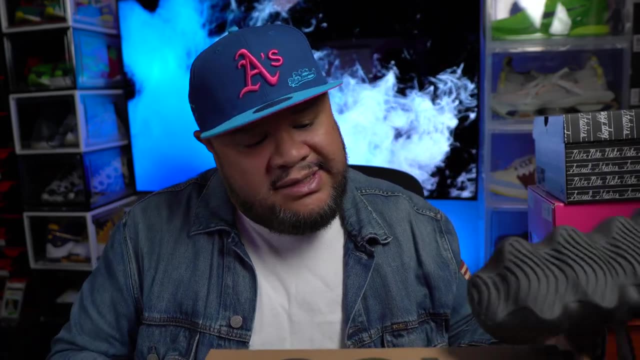 out just for y'all to see this, because it's unbelievable what I can see, why Kanye wants to leave Adidas. So these are made in Germany. I think both are made in Germany. This is the Utility Black. All right, Now let's just look at it in detail. It's, it's similar to the Utility. 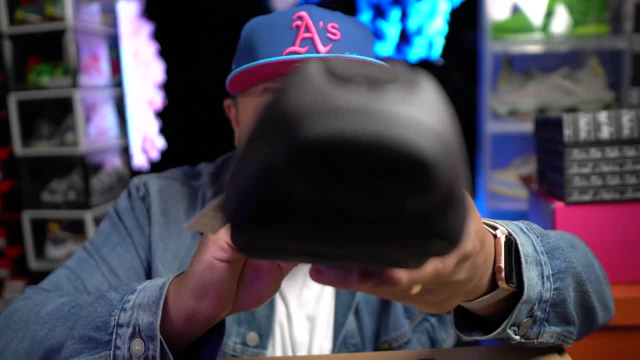 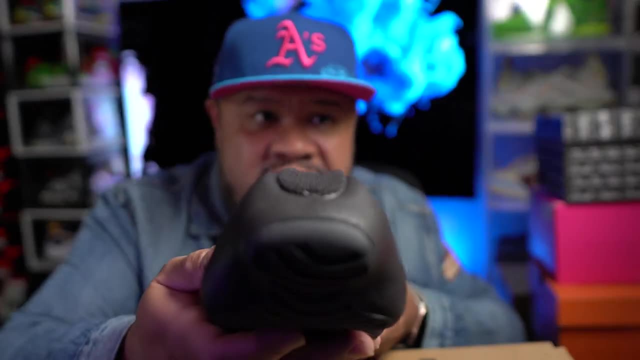 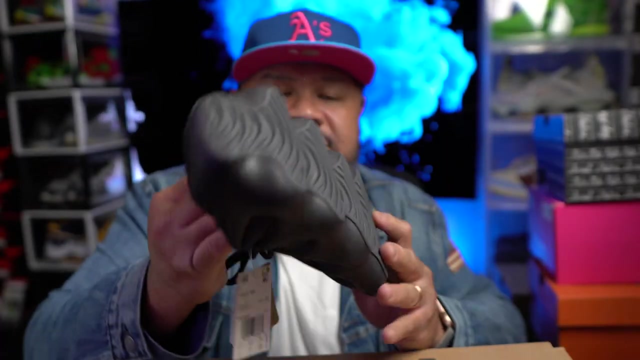 Black 500.. So you got all this. The heel is very, it's not focusing. Yeah, The heel is all all black. That nice, that nice slate color, Very nice. I like these. This is dope. So if I were to keep one, I'd keep this one. But see the top, the upper, same thing. 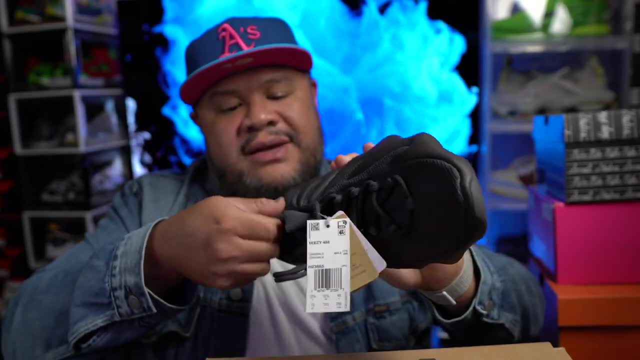 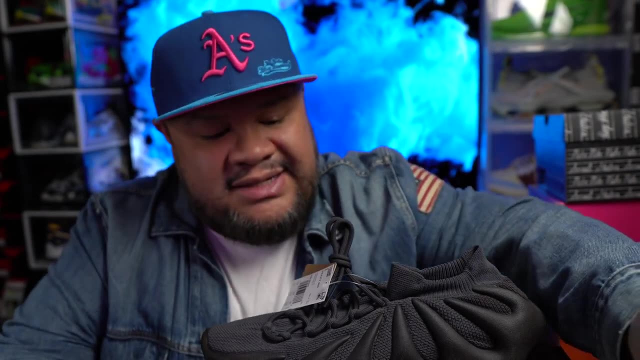 I mean y'all, y'all. I did three videos in 450s, or two or three videos, I don't know. I like them a lot. They're cozy, They're comfy, Not a bad shoe at all. Next, mind you, this is going to be a quick. 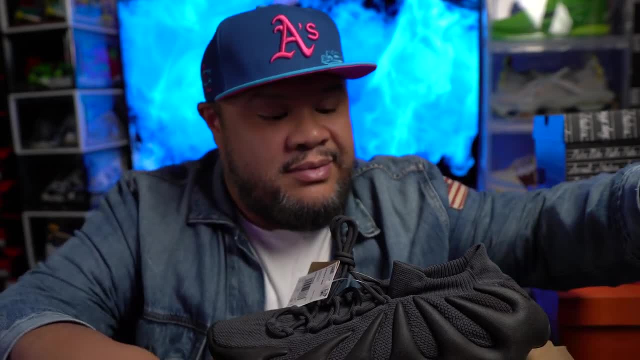 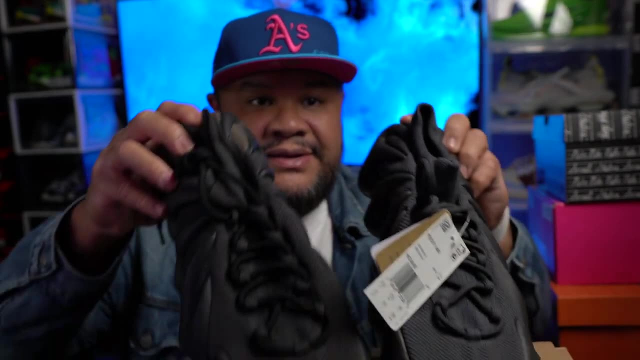 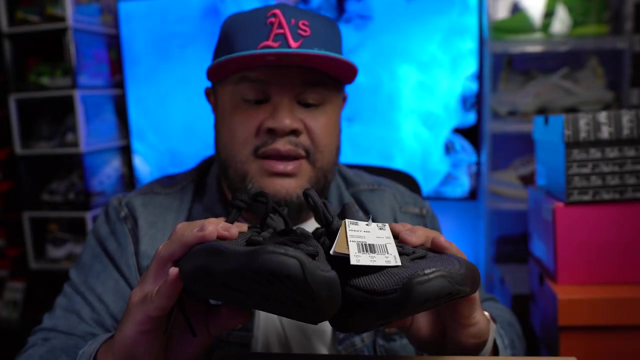 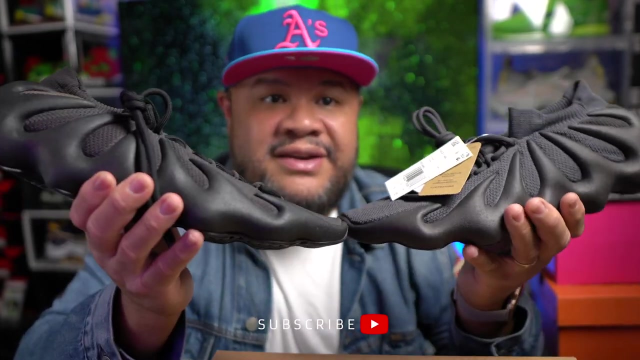 video because I just wanted to do it to prove a point about what Adidas is doing. So here is the 450 slate: The uppers are identical in blackness. The laces are identical in blackness. The creepity crawly claw thingy on the side that's supposed to give you all the 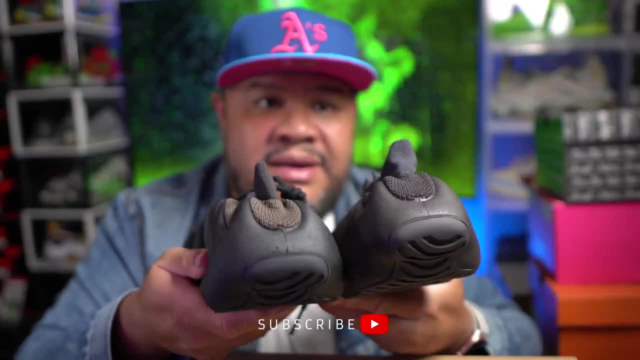 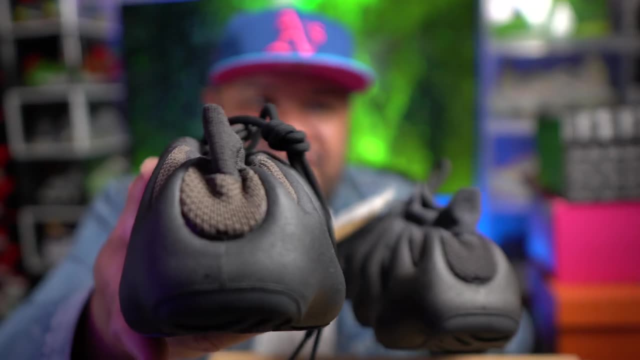 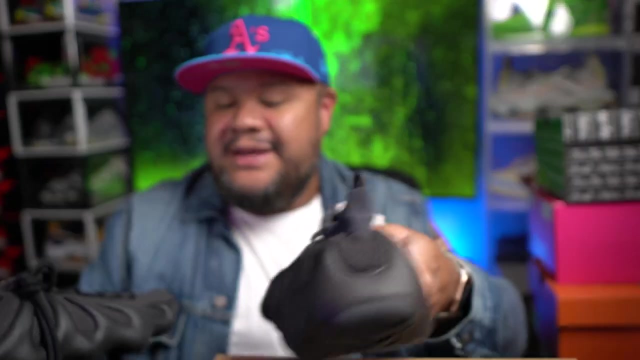 support are equal in blackness. Right. here's the difference. There's right here On the slate: it's like a brown. On here it's all black. That's it. Kanye says he did not approve these colors because they're stupid colorways. That's stupid. This is the 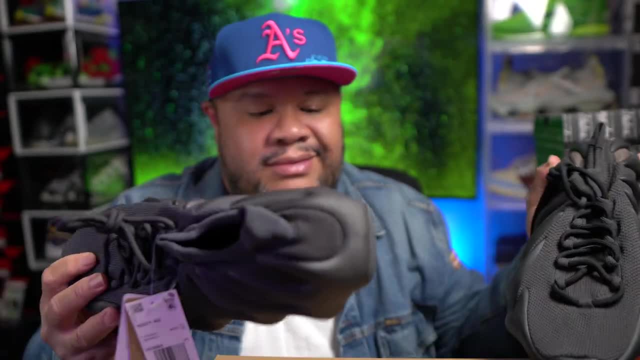 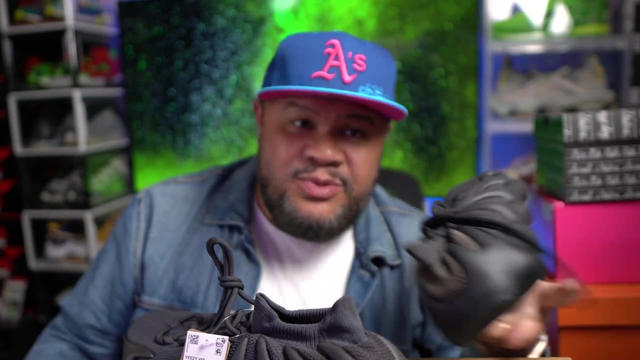 dumbest thing Like: honestly, if you're going to go all black, why? why would you put some? this is like I know what happened here. I'm going to tell you this is my theory. It costs more to make this one because it's essentially too, too knit. 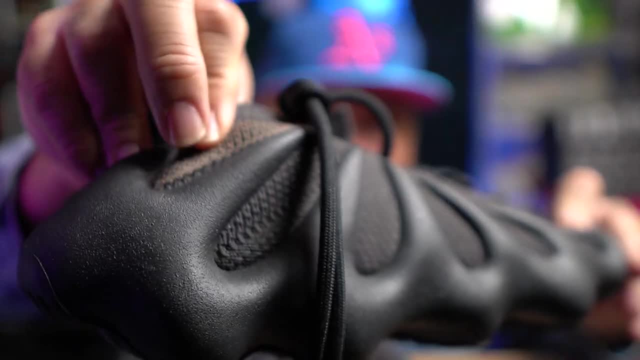 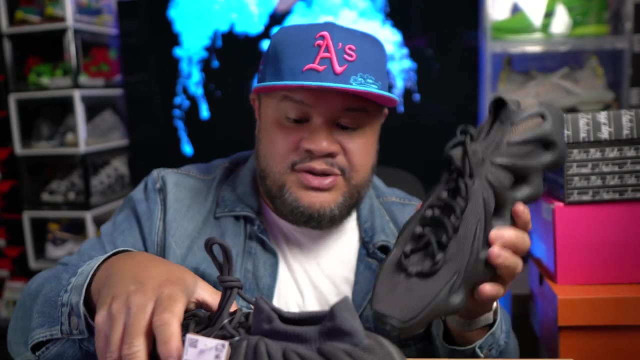 too, pieces of knit fabric, If you could see that these are knitted together back here. So it had to put a little extra into the upper. You have to get two pieces of fabric and obviously, quality control. blah, blah, blah. These have very good quality control. You don't really see. 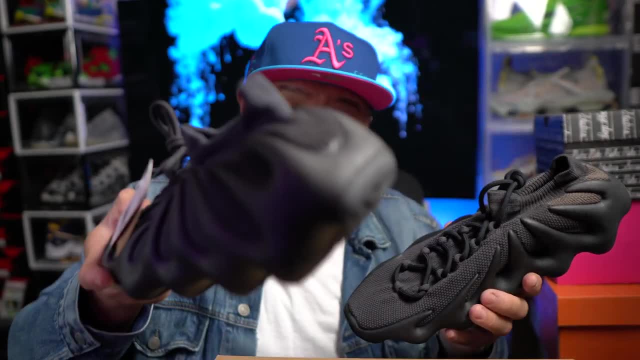 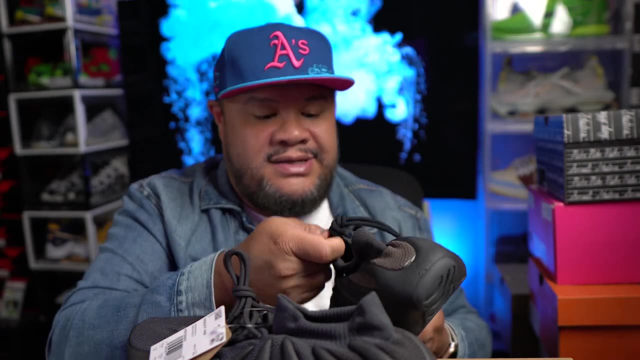 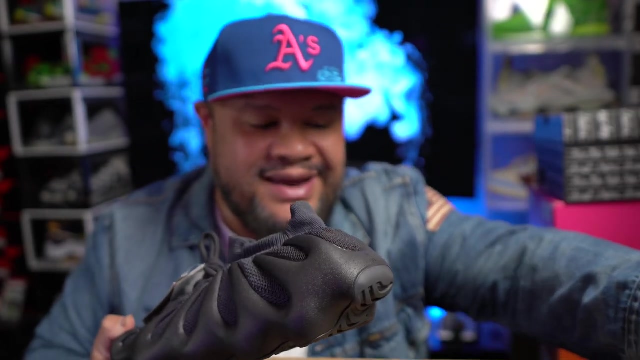 many glue marks and stuff like that on these. They're pretty good. This is all one piece, I'm assuming. I'm going to assume that. So, oh man, I Adidas is really on something right now. when it comes to Kanye- And I think it's, it's more or less- they're like Hey look. 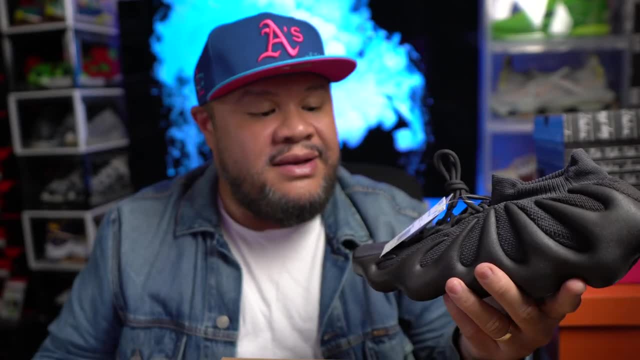 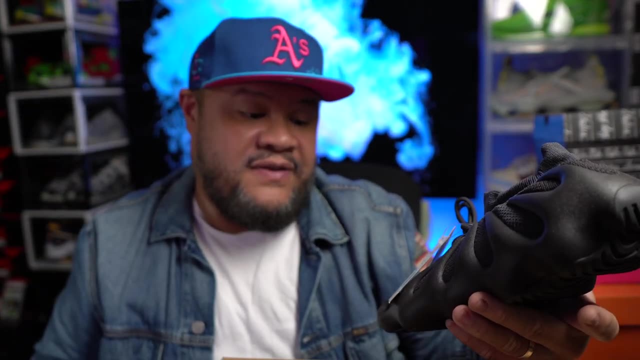 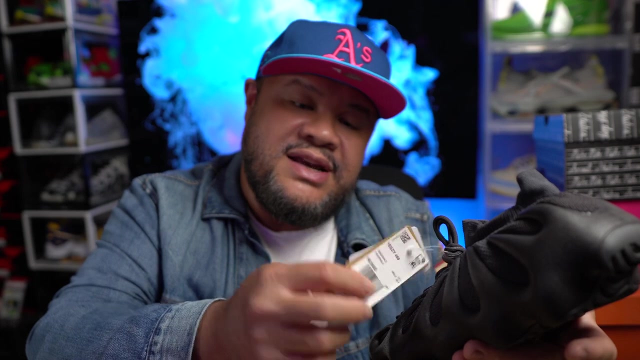 you in contract with us till whenever, and you can go wherever you want whenever you want. So it is what it is, but I'm like befuddled here And this is interesting- I bought a size third. oh no, it's 13 US, it's 12 and a half. Okay, Nevermind, That's UK size and 12 and a half. 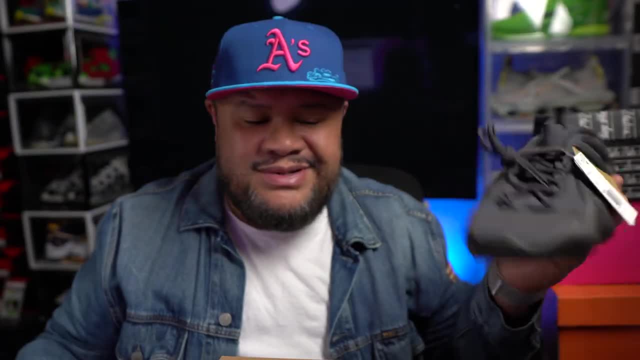 Nevermind, Yeah, But these, these, these are dope. I think I'm going to just keep the black ones. I don't need to hit a Brown, It doesn't matter. I'm done with these shoes. This is the last pair. 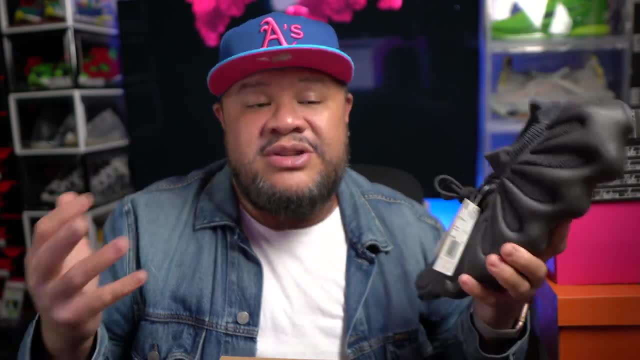 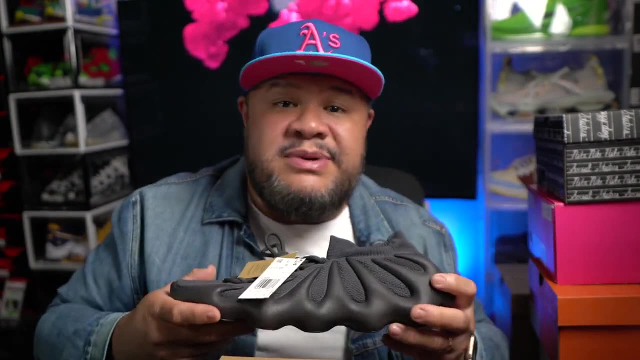 I'm actually going to buy, unless they come out with something like multicolor. uh, that looks dope, like they did with five hundreds to number. five hundreds always came out in these bland ass colors. So, yeah, that's. that's basically all I got. And look what I copped on easy day I got. 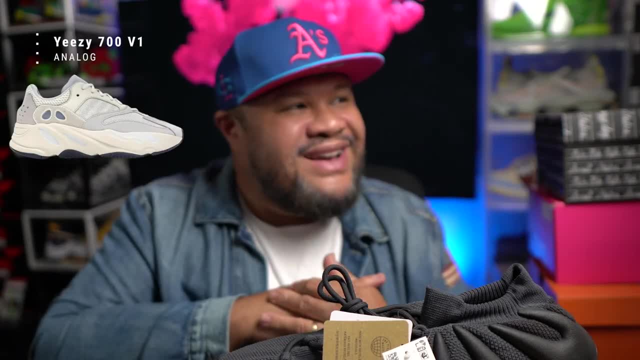 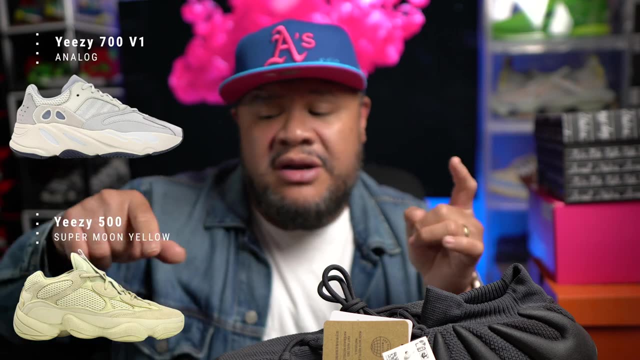 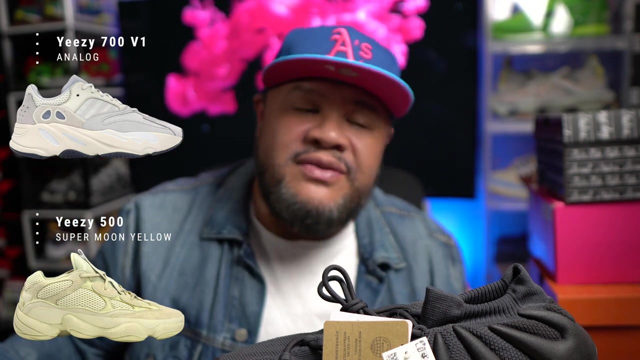 the analog 700 and then I got um, uh, five hundreds, which I always wanted. Um, they should be here tomorrow actually, And those are super dope. I um only could get them in a size, So I could have gotten more of easy supply. They were kind of sitting there. I tried to get a 12 and a. 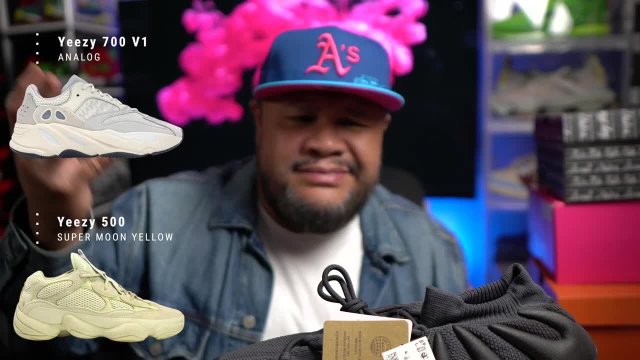 10,. uh, I got to squeeze my foot into that 12 or try to sell up to a. if they're worth anything, I don't know. I have to look at the- uh, the pricing on that 500.. That's one of the better. 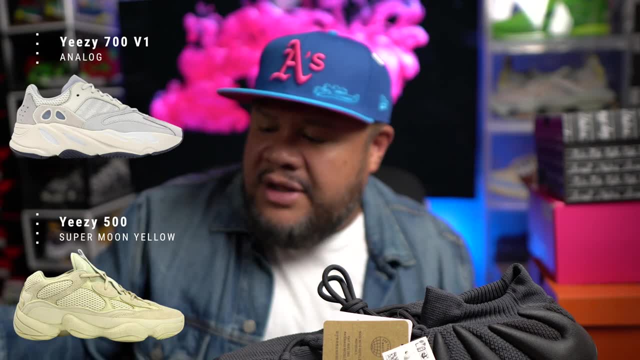 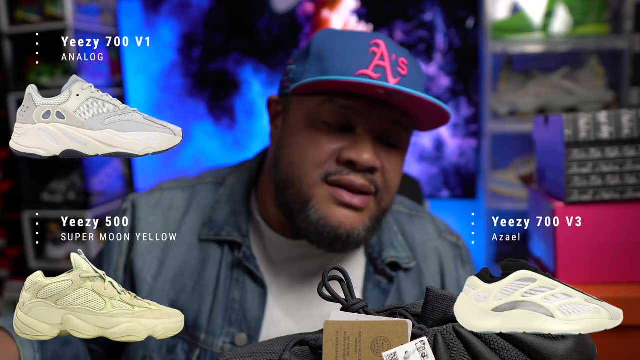 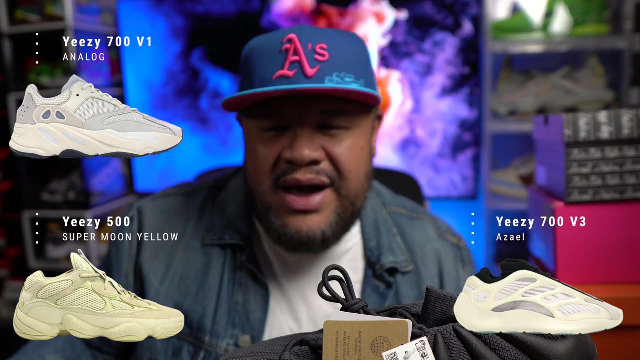 colorways. And what else am I waiting for? The first model of the Yeezy uh 700 V3. Those are coming in. those I like a lot. Um, I do love the 700 V3 now that I know how it fits and I wear. 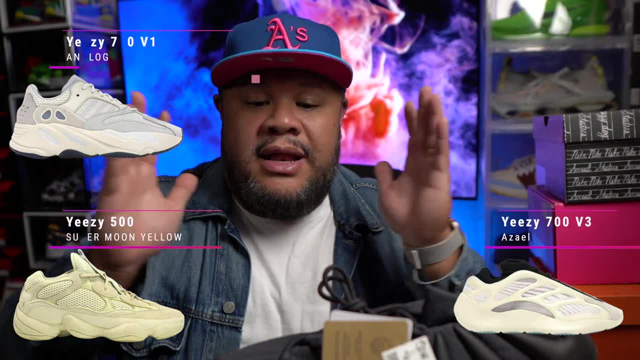 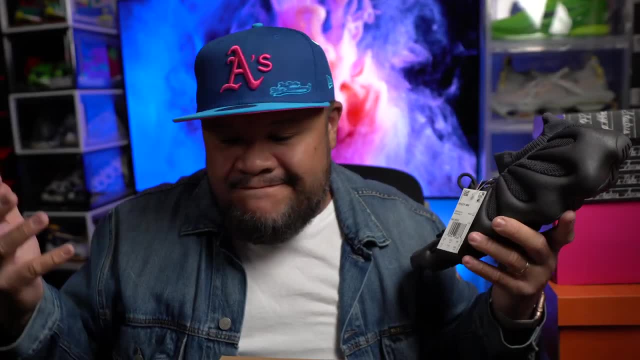 those types of shoes Frequently, So that's all I got like. subscribe. Tell me what you think about this colorway, the black on black, easy, And um, yeah, we'll check you in the next one. Let me know how your. 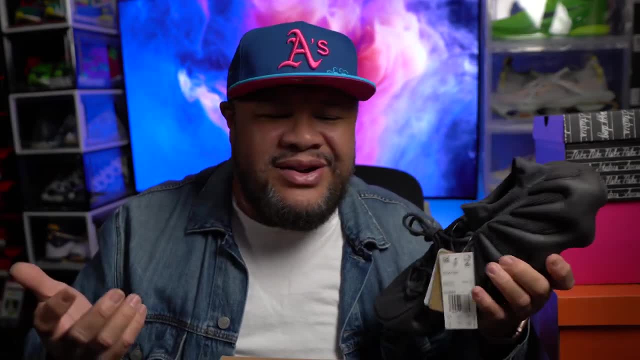 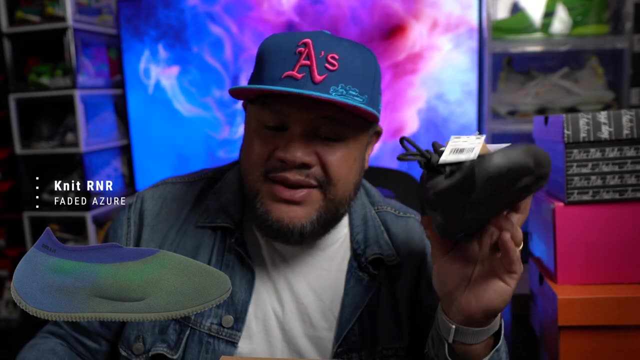 Yeezy day went in the comments below and tell me what other colorway I mean they released. I mean I do like that knit runner and I want a pair of those. I actually they're not going for that high Like the other. the older models are going for like $600 on resale. Uh, there's not many. 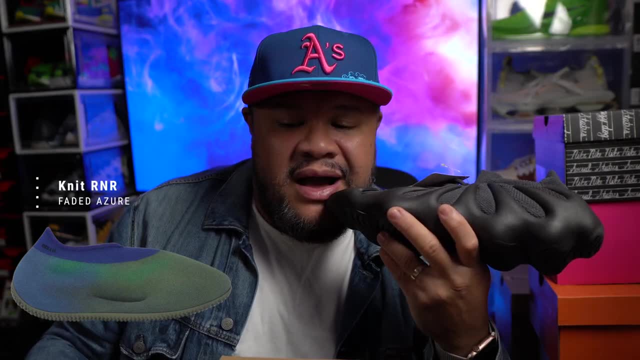 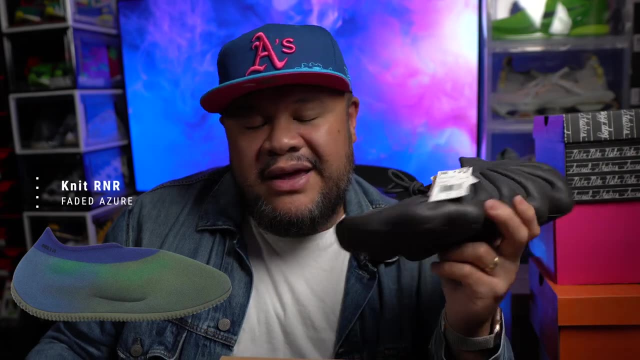 of those out there. So, long story short, I'm like I want to, I want, I want the pair of this colorful pair, Cause I actually have a fit for the winter that goes with it, The stone Island jump off that I got And, um, hopefully I could get it. I put in max, I would pay for it, I think. 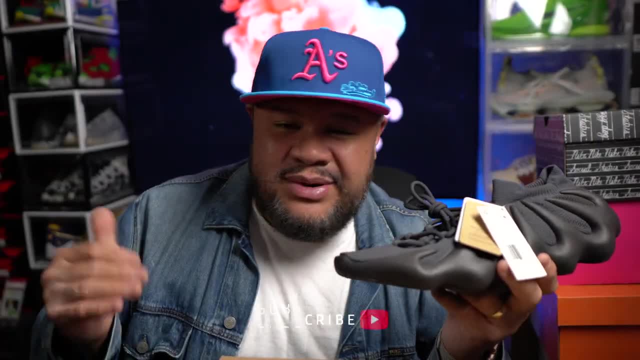 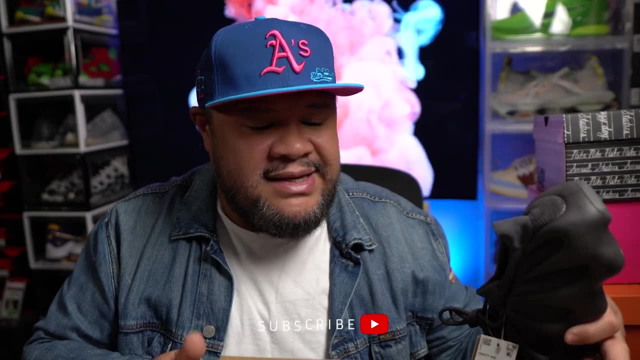 around two, 80, I think I put in so it'll. it'll hit that when, when people start getting their packages and realizing they don't want that shoe, but yeah, like subscribe, tell me what you think of these. uh, Yeezy and the Yeezy day overall. Tell me how you did. If you went for anything and um, I'll check in the next one, Peace.